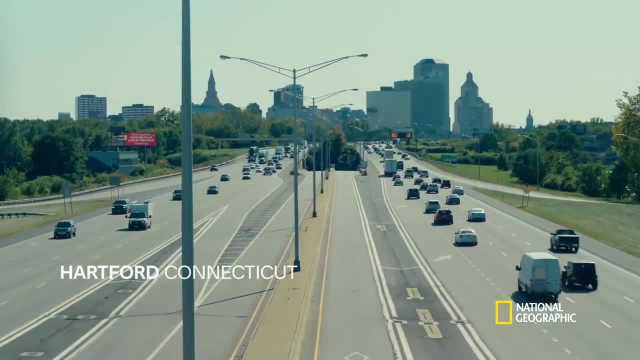 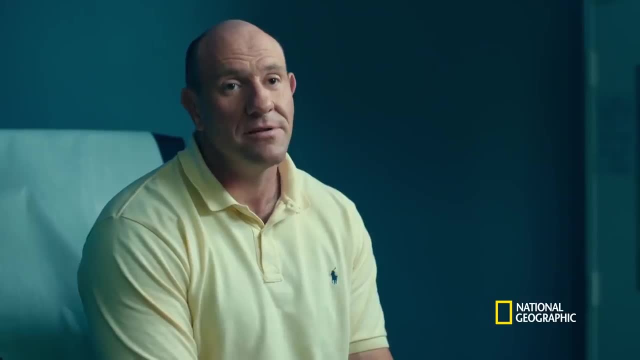 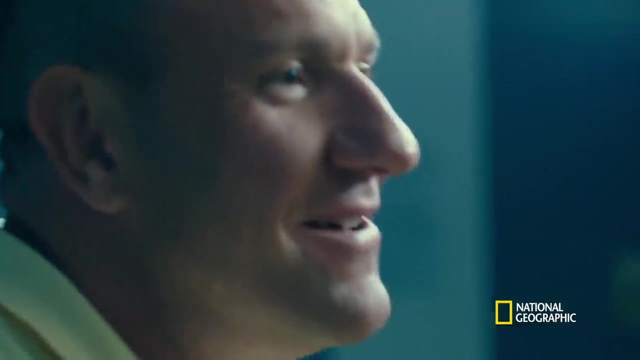 I think some of the damage I did is probably permanent as far as an enlarged heart. I don't want to go back and bodybuild. I'm not looking for that, I'm looking for you. know how long can I live right? I mean, if you look around this office, who's here? It's old men, It's. 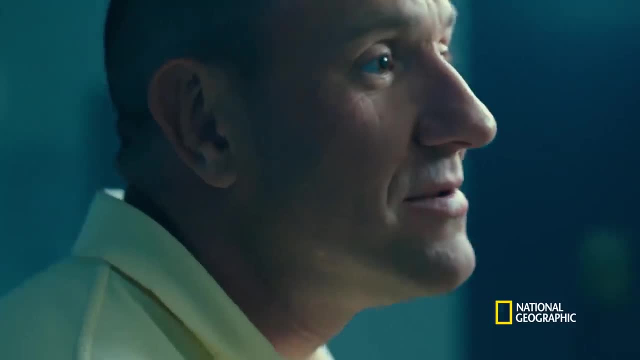 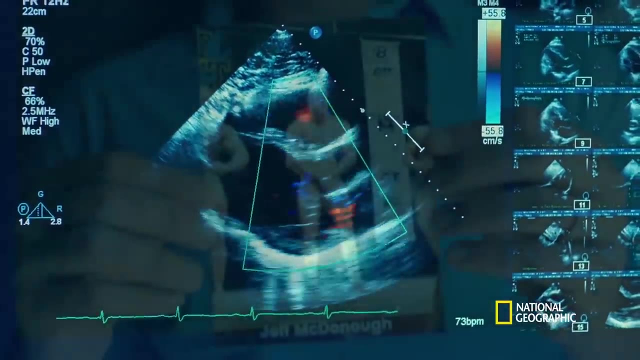 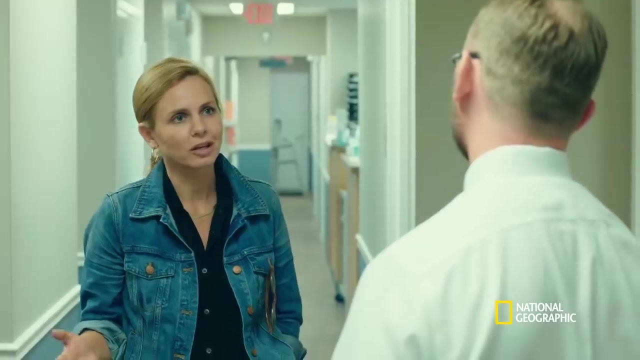 like: why am I here? I'm freaking, 37. Something's wrong, right? Jeff has been under the care of a cardiologist for the past year, ever since doctors treating his steroid infection also discovered signs of heart failure. So, doctor, because Jeff took testosterone for so many years, now his body doesn't produce it. naturally and he actually has to take testosterone to stay healthy. This is the unfortunate irony for guys that are looking to become superhuman per se. Now they end up in a point where, again, they obliterate their body's own ability to produce. 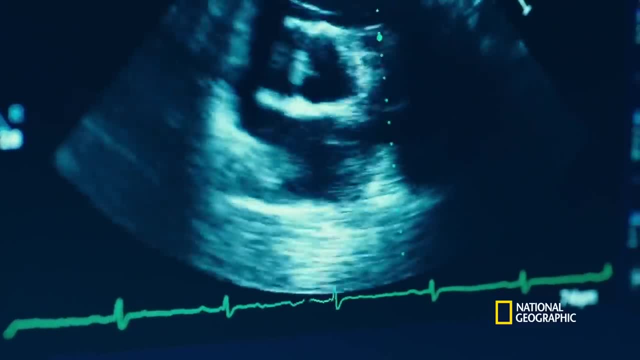 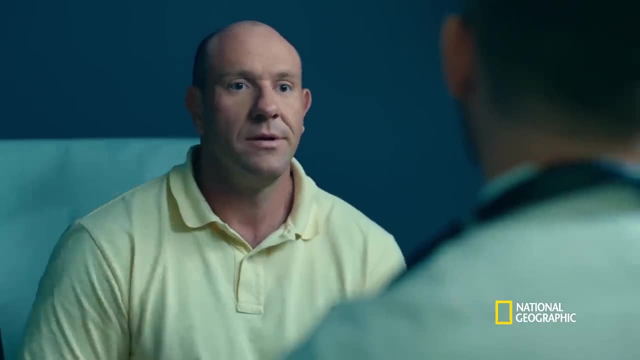 testosterone. Today, Jeff will be getting the results to see if his heart has bounced back to normal. So there's two main things that we're evaluating with that echo. One is your systolic function, which is the squeezing function, and that was the one that was mildly reduced last time. 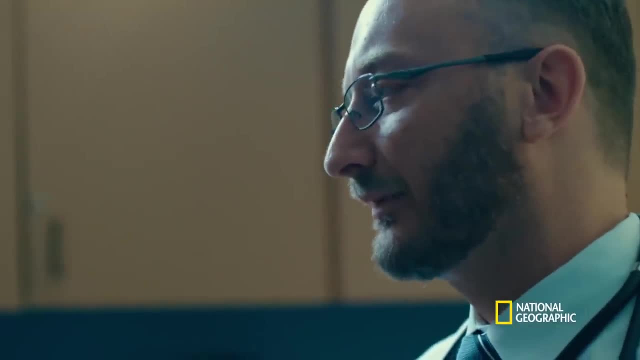 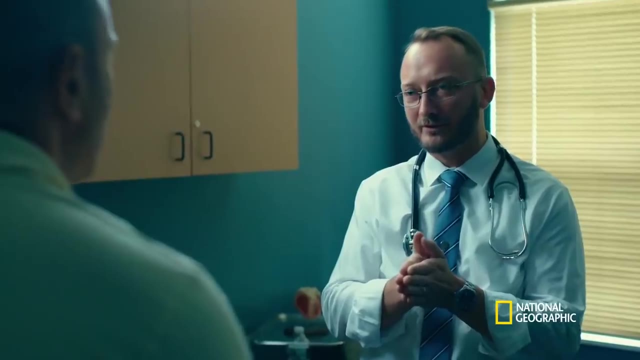 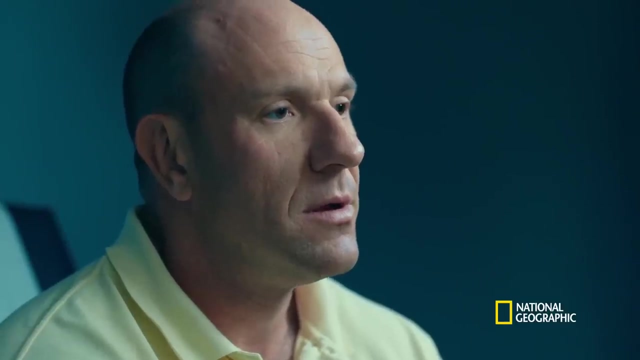 you were here, That actually does not look significantly different. Okay, so it still looks a little bit sluggish, But there's another parameter that we look at, which is the relaxation function of the heart Right, And it's also quite abnormal. last time you were here, That looks significantly better. 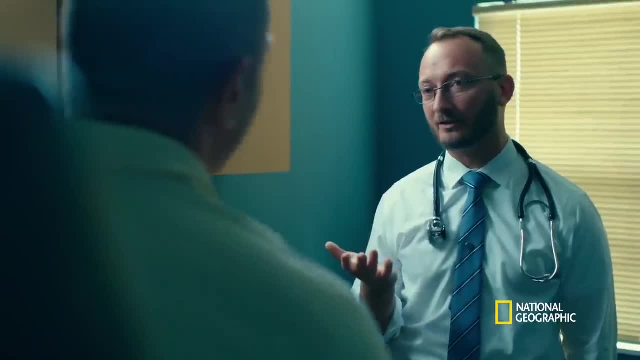 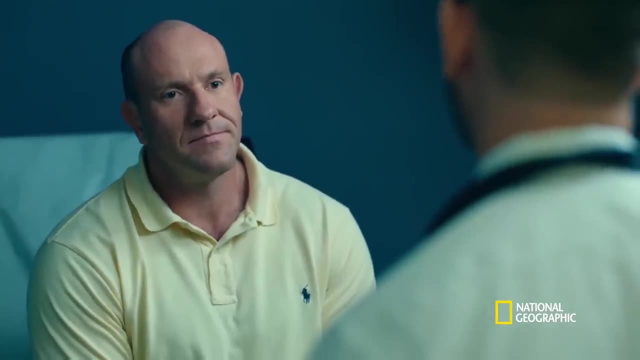 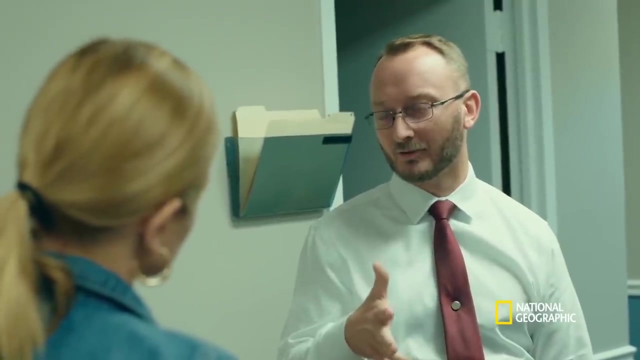 Okay. Okay, You know we're not at the point where I'd say: your heart looks normal, unfortunately, Right? I think you should sort of get your mind around the fact that you're probably going to be on long-term medication. I worry about Jeff's longevity. His heart actually hasn't bounced back to normal And 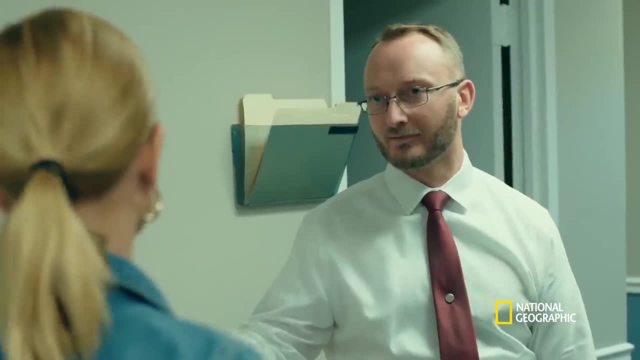 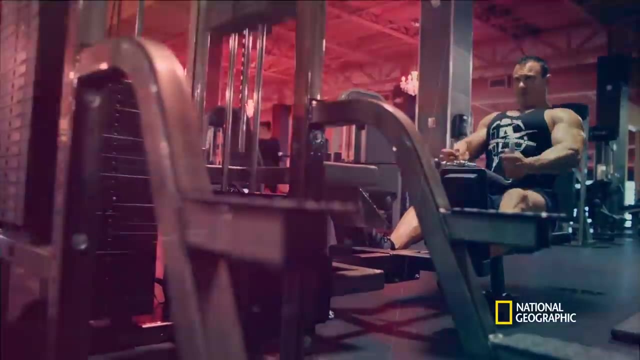 the longer we see it. that sort of suggests that something permanent has happened there And if he started taking steroids again, Not exactly That's a pretty good outlook. We've heard from a lot of people that say that there's a safe way of doing this. The 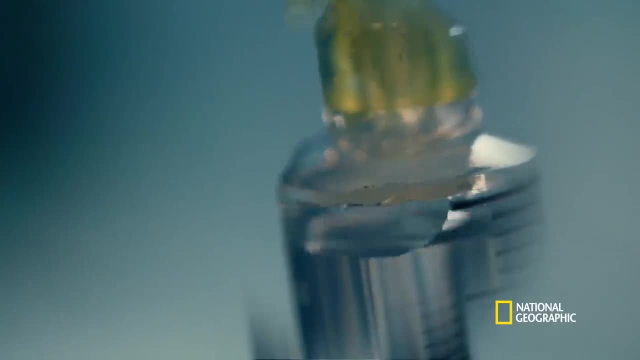 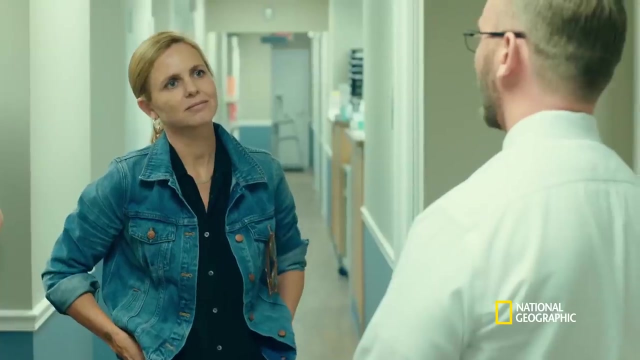 people that have gotten hurt is because they didn't know what they were doing and they were taking too much, But there is actually a safe way to do this Right. What do you think? I think those people are kidding themselves. The best data that we have are autopsy studies. 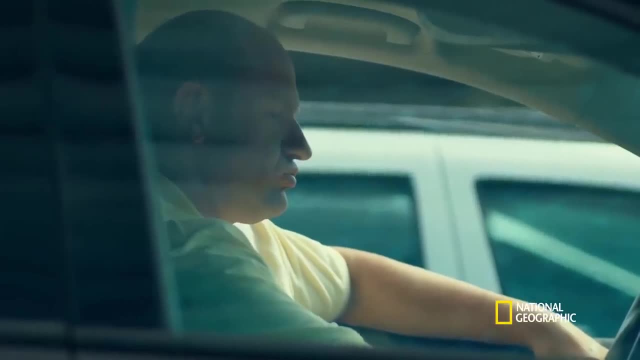 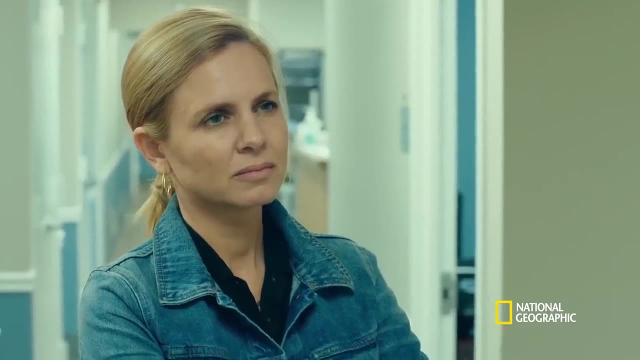 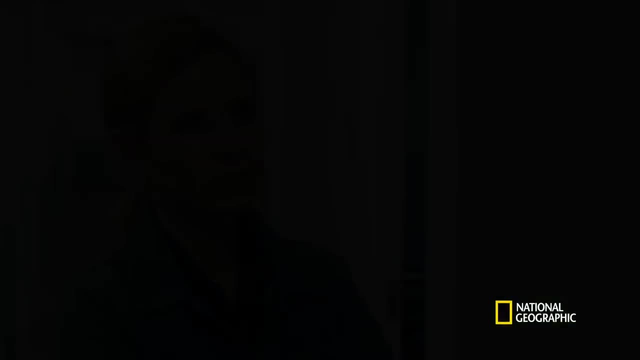 Yeah, How, what? how do have we made a decontaminated word? Isn't life getting 300 months easier In America? it's killer We're taking there's being able to be allergic to the eye for 30 to 40 minutes every day. 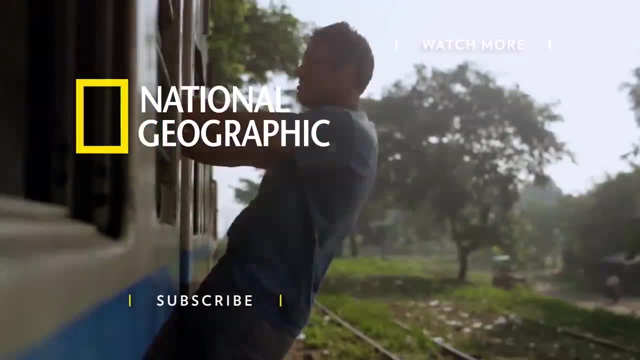 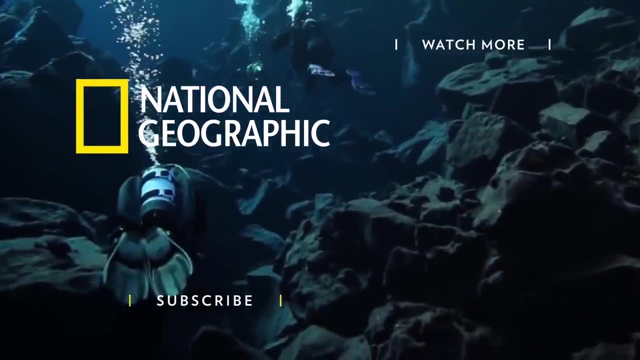 God be with you. Thank you very much. That's been excellent. Yeah, All the best. Thank you for this assistance. Thank you, Have a wonderful day. How the hell did she cry right out there? Yes, Yeah, The baby's almost to the sea. Yeah, you know like you know. so it'll get moving very little by little, But in theüll I respect that sort of production Absolutely. I appreciate it. Yeah, Going to the bowl to get you a hot sauce. No, thanks How you doing. 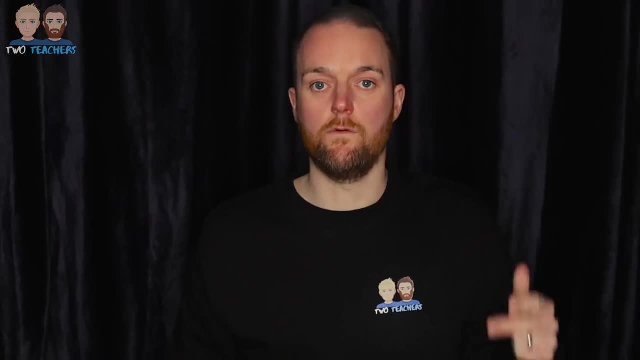 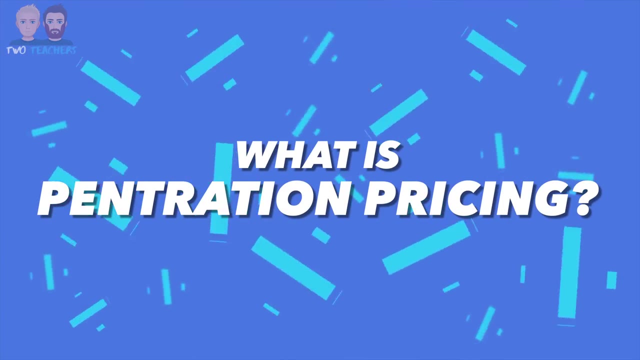 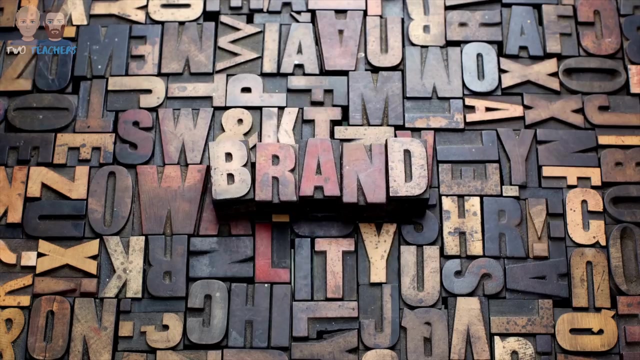 Amazon, Virgin Media and Disney have all used penetration pricing to establish a foothold in new markets. So what exactly is penetration pricing? Simply put, it's when a business sets its initial price really low in order to gain market share and establish its brand. Imagine: 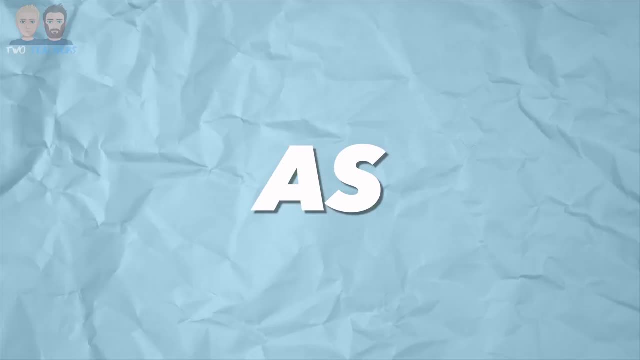 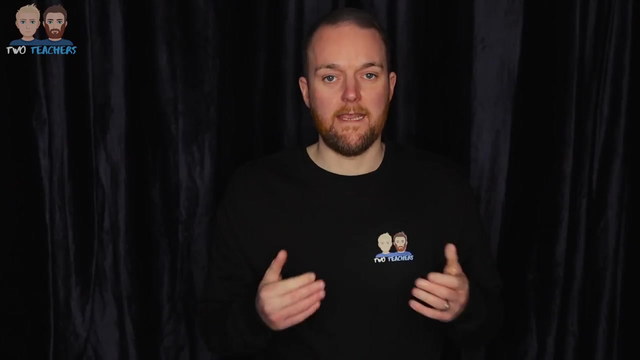 you're launching a new product and you want to gain market share as quickly as possible, You could offer a low introductory price just to get customers using your product or service and make it easier for them to try it out and become interested in the product. Once you've then built. 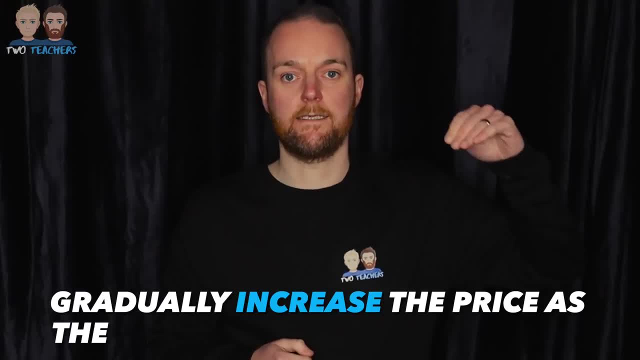 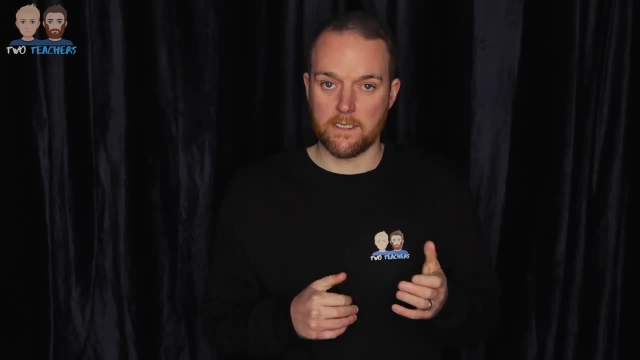 that base of customers. you then gradually increase the price as they become loyal to the brand. In 2020, Disney entered the crowded UK streaming market with its own platform, Disney Plus. At this point, it had a zero percent market share and was competing against major players like Netflix and 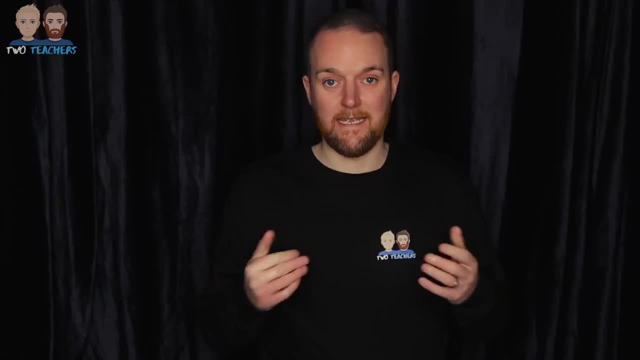 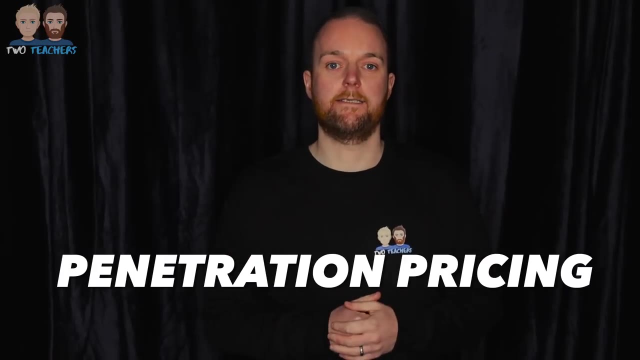 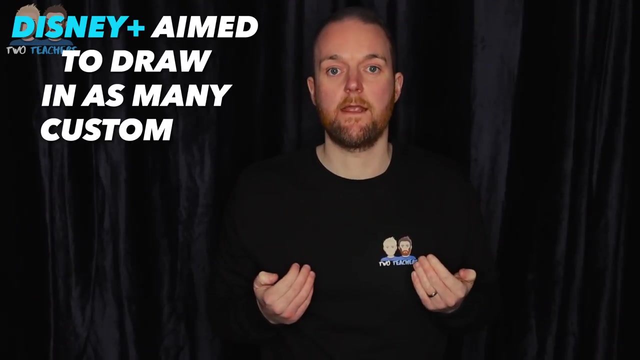 Amazon Prime that were already dominating the market, Disney needed a way to stand out and get new subscribers. One way they did this was with penetration pricing, By offering a low monthly fee of $5.99 along with a free trial. Disney Plus aimed to draw in as many customers as possible with a more 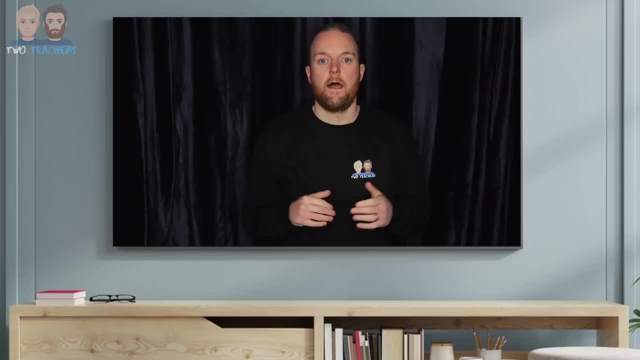 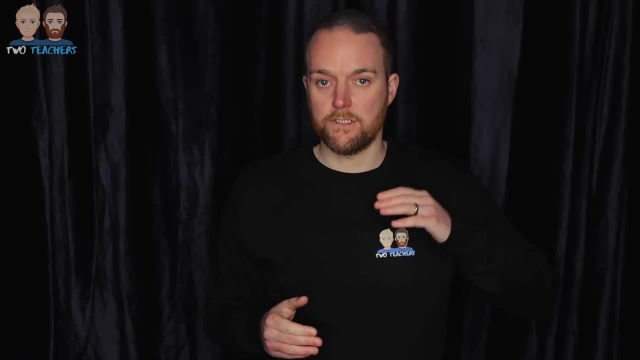 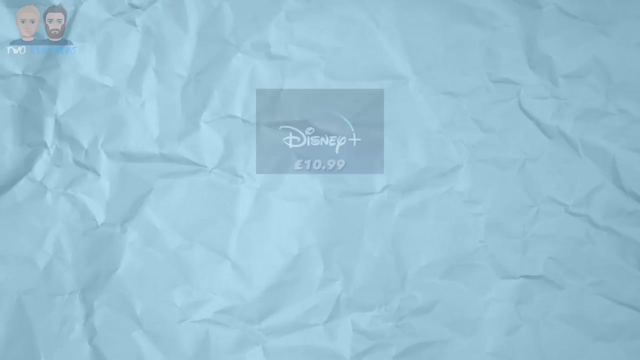 new customers into a more attractive product. This was the first time Disney Plus had ever turned customers into long-term loyal customers. After the successful launch of Disney Plus using penetration pricing, the company shifted their strategy and gradually began raising their prices, first to $7.99 a month and now an expected rise in 2023 to $10.99 a month, Making their prices